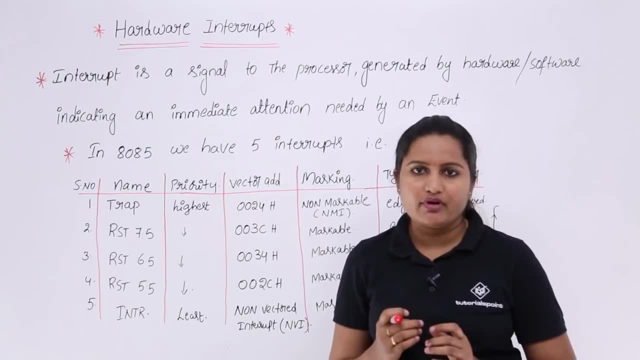 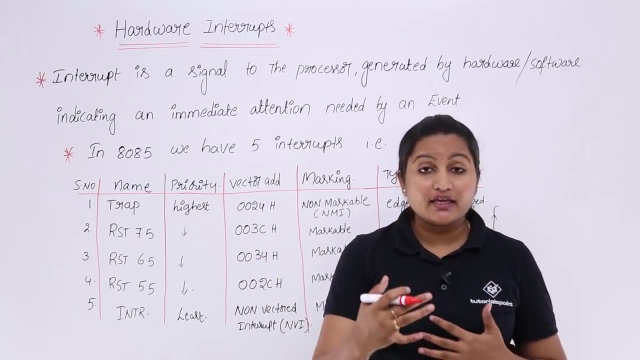 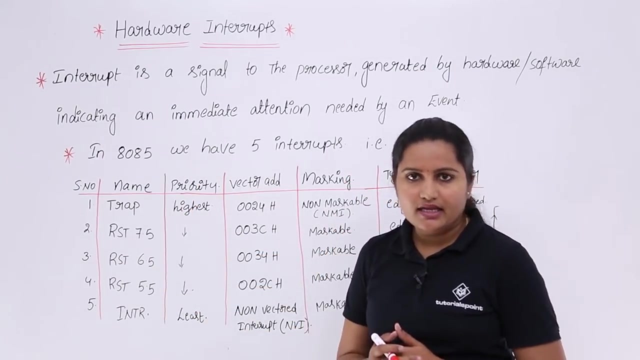 device connected to this processor that it requires immediate operation, So that is called as hardware interrupt. So here in 8085, we have 5 types of interrupts. So here we are having that interrupts here. So according to the priority I return these interrupts. So trap is first interrupt and RST. 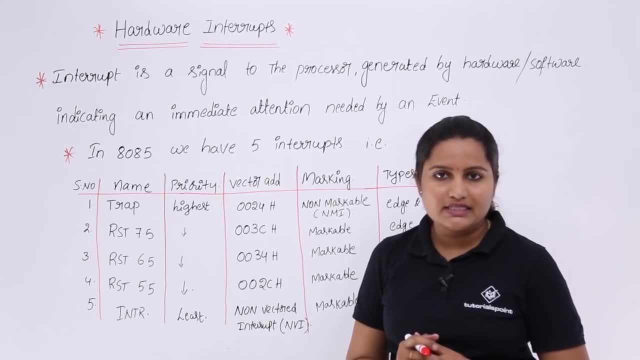 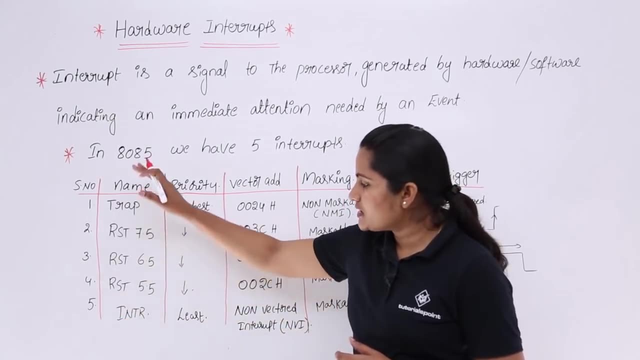 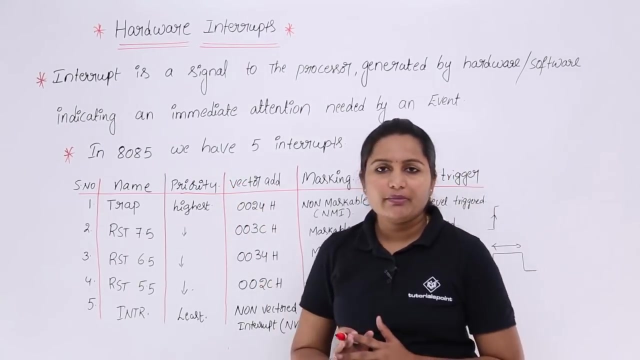 7.5, that RST corresponds to reset 7.5, RST 6.5, RST 5.5 and INTR interrupt. So these are all the 5 hardware interrupts in 8085 microprocessor. And coming to the priority trap is always given for. 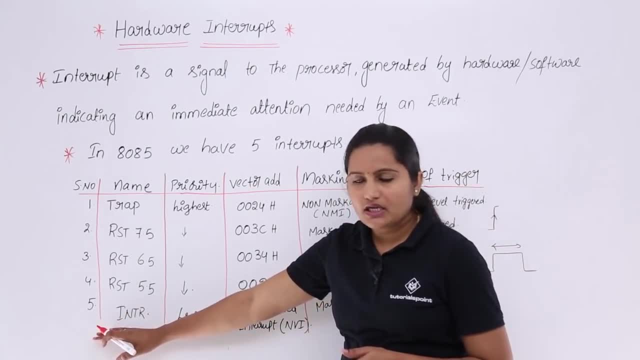 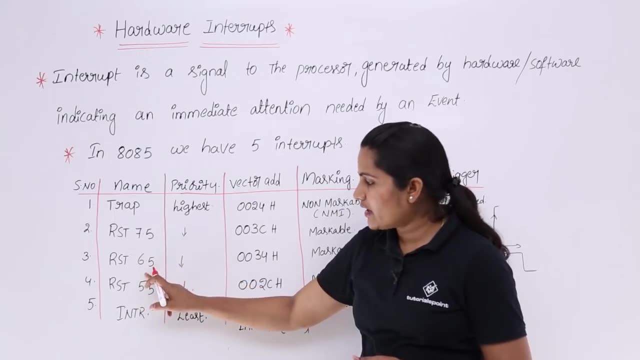 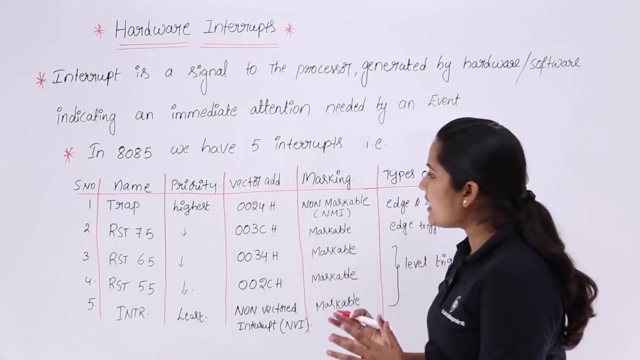 highest priority and lowest priority is INTR, So remaining, I return in that priority only. that means after TRAP you are having 7.5, after the 6.5 and 5.5, and least priority is given for INTR. Then next coming to vector address: the vector. 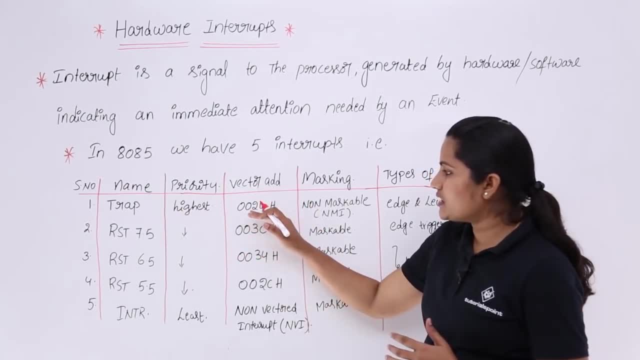 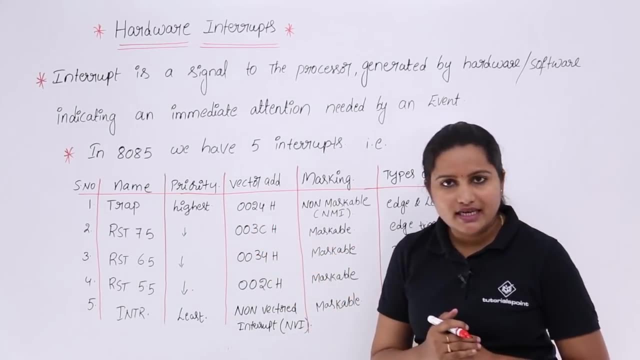 address of TRAP trap instruction is 0024H and the vector address of RST 7.5 is 003CH and for 6.5 this is 0034H. These addresses are very important for your technical point of view. technical exams point. 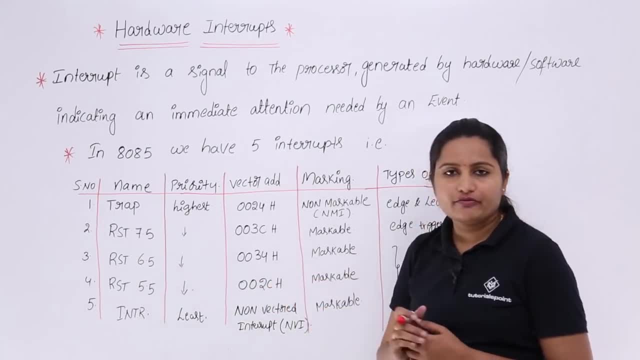 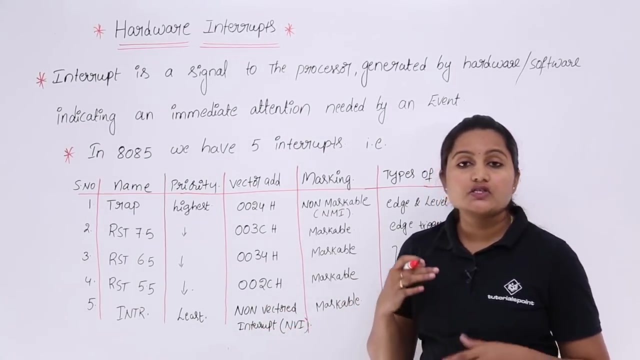 of view and for the vector address of 5.5, RST 5.5 interrupt is 002CH, So here INTR is having no address. that means this is a non-vectored interrupt. So this point is also very important. 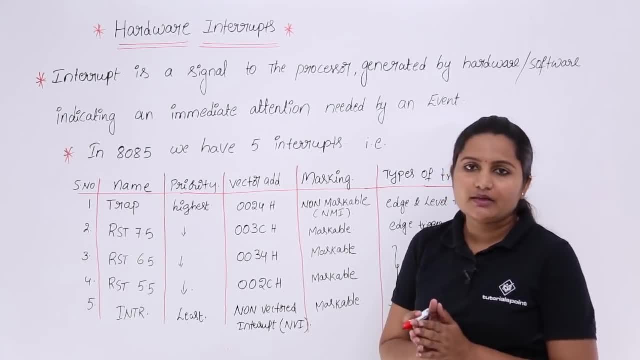 point We are having. how many non-vectored interrupts are there in hardware interrupts? So this is a non-vectored interrupt. So this is a non-vectored interrupt. So this is a non-vectored means. So we are having one non-vectored interrupt, that is INTR. So here generally, 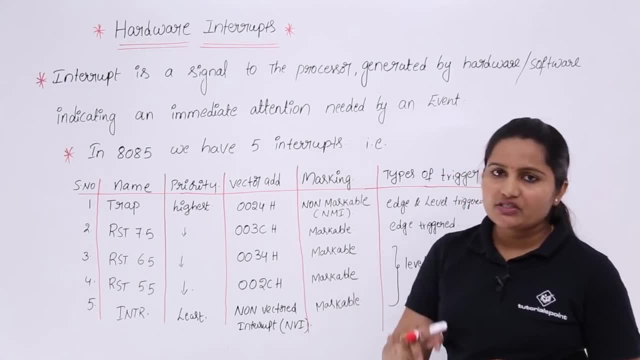 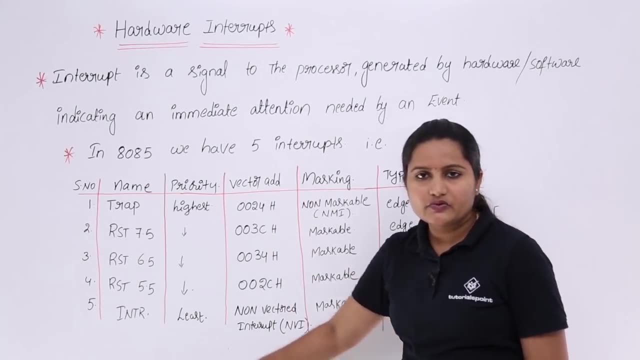 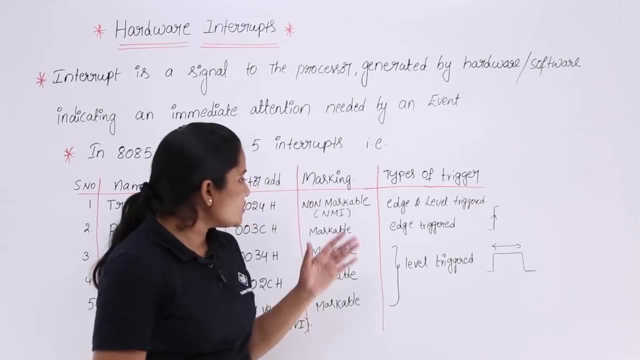 hardware interrupts are classified into two types, that is, vectored interrupts and non-vectored interrupts. Under vectored interrupts, we are having this four. under non-vectored interrupts, we are having this one fifth one. So coming to masking, masking means disabling, So here this TRAP is a. 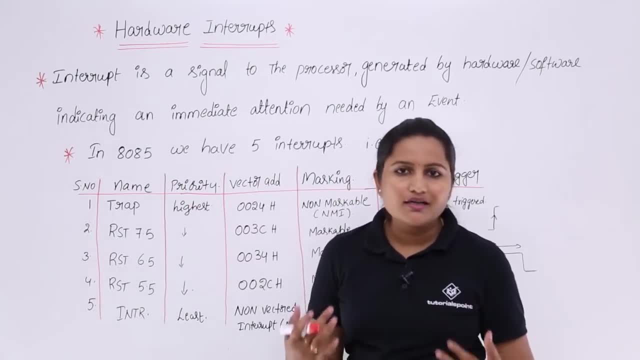 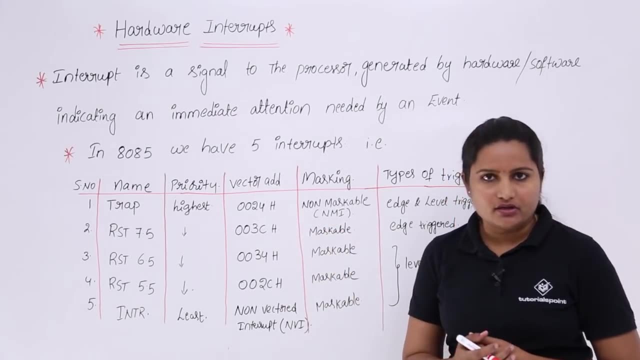 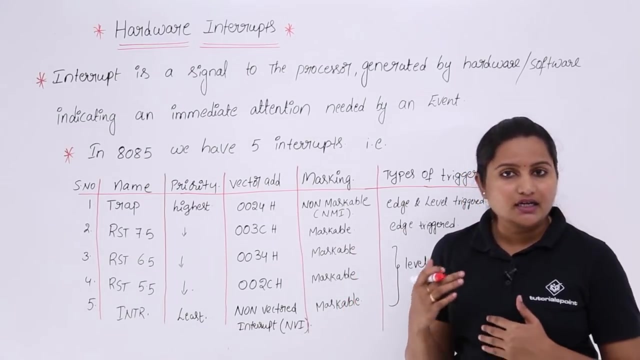 non-maskable interrupt. So that means we cannot disable. So always it will be in enable condition and remaining four are maskable interrupts. that means, So only TRAP is non-maskable interrupts, remaining four are maskable. that means we can disable by executing DI DI program. 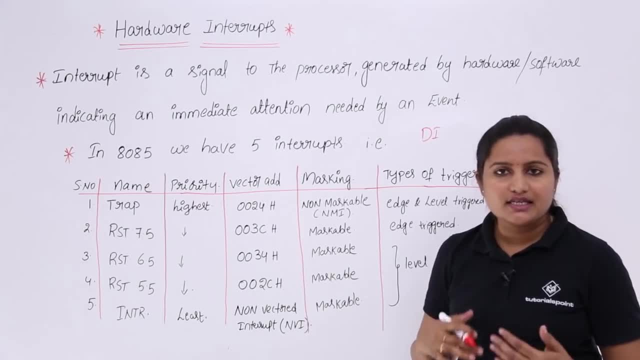 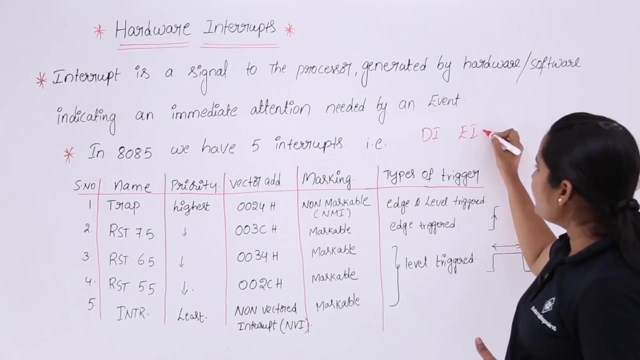 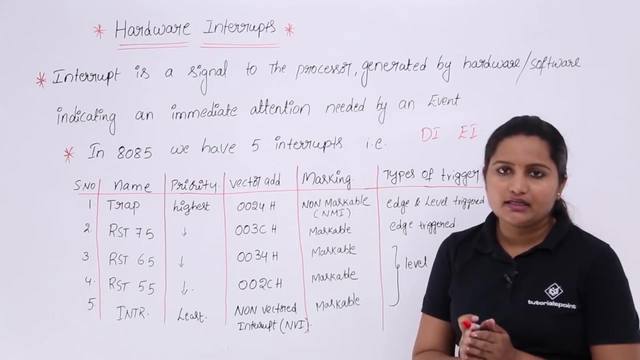 that means disable instruction command. we can disable these interruptions, So non-vectored interrupts. So now and re-execute by using execution of EI. that means: So these four are the maskable interrupts. that means we can disable that interrupts by executing DI. 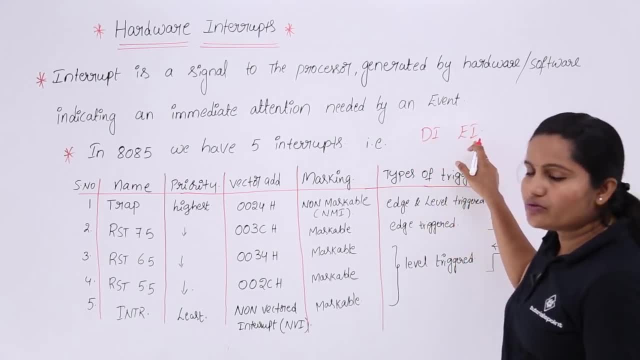 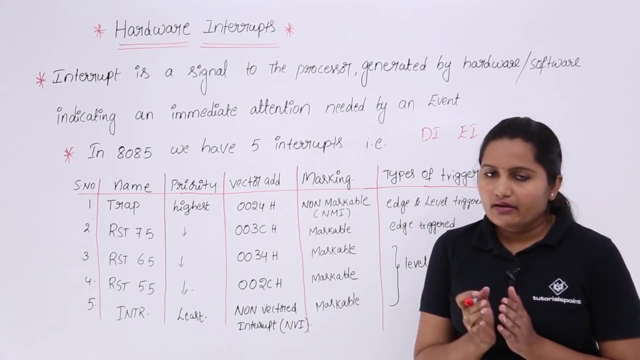 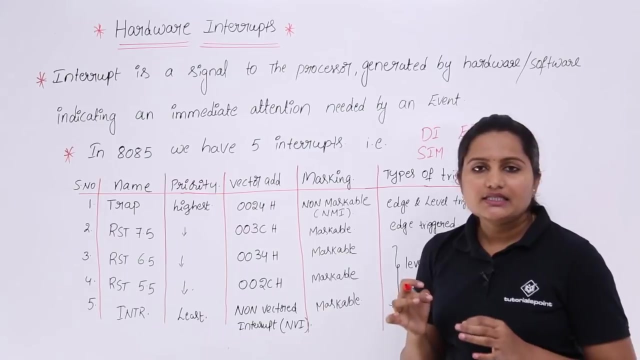 disable instruction interrupt and re-enable by using execution of EI: enable interrupt. So now, so we are having a set by using SIM, set interrupt mask. this is also one command. So we are having set interrupt mask. So by executing SIM also we can masked these. 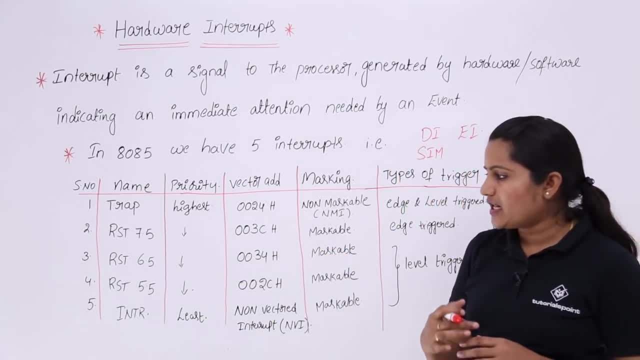 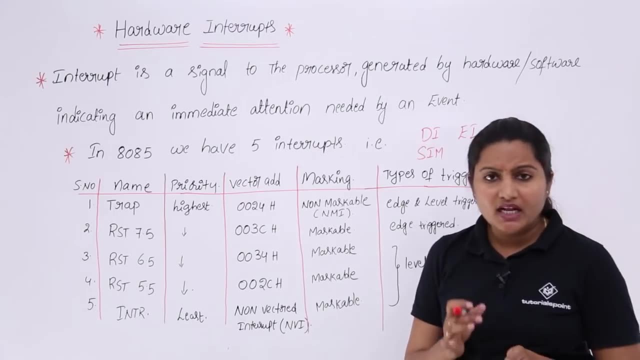 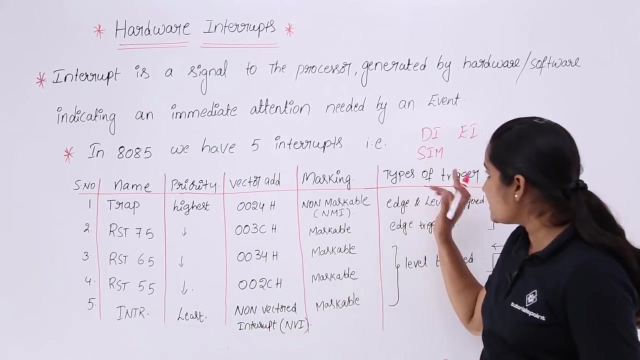 three interrupts. that means RST7.5,, RST6.5,, RST5.5. we can mask by using SIM also. That means SIM means set interrupt, mask. so but we cannot mask I and TR by using SIM, by using. 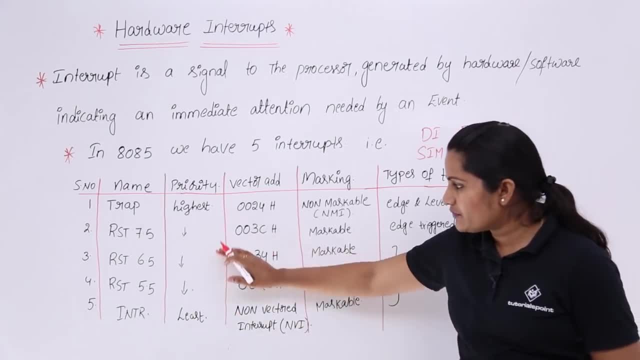 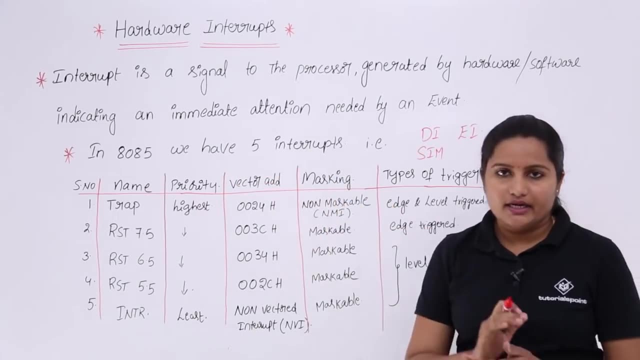 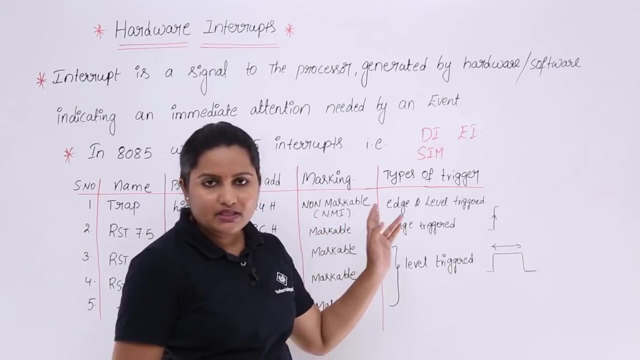 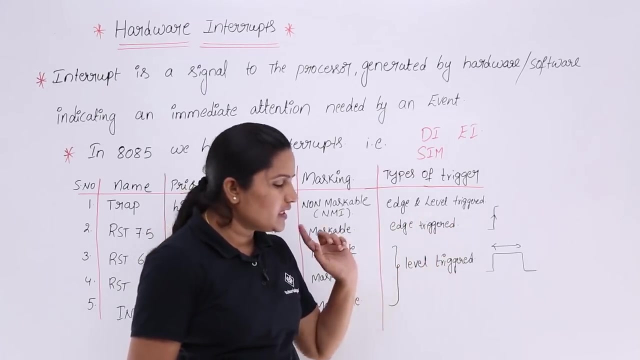 DI and EI and enable these four interrupts, but trap is always it will be in enable condition. this is a non-maskable interrupt and, coming to type of triggering, so these are edge and level triggered trap interrupts are edge triggered as well as level triggered and rst 7.5, only edge triggered. 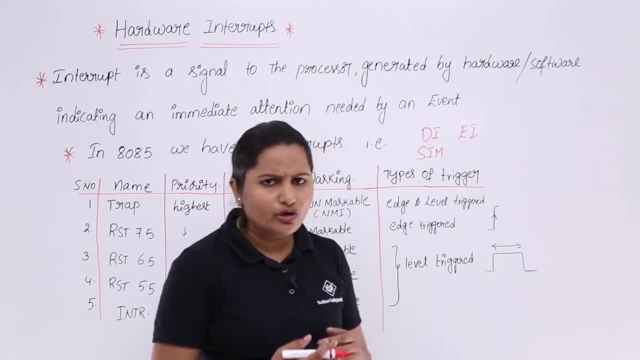 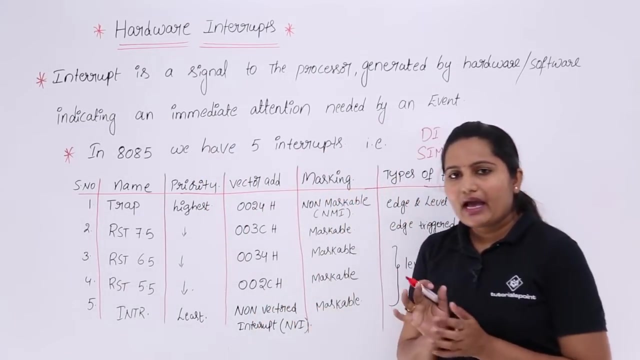 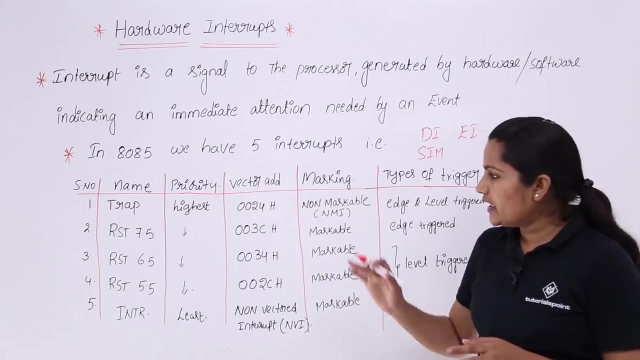 remaining three are level triggered interrupts. you know about edge triggering and level triggering, so positive going ah edge of clock will enable these. ah means edge triggering, so level, if you consider that is called as level triggering. and coming to here they may ask questions like this: what are the ah, non-maskable ah, vectored interrupt? so in the interrupts you are having non-maskable.